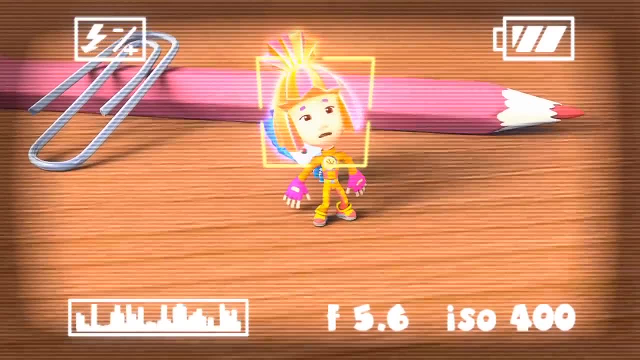 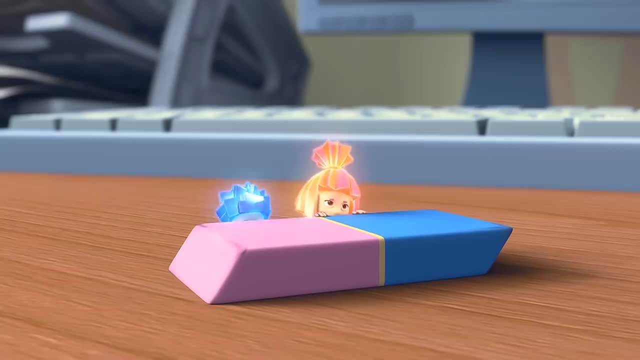 Hey, what about your promise? What promise? To never take a picture of us? We're a secret. Stop, Hey, relax, I'll delete them all later. Tom Thomas, stop this right now. I won't until I get a photo of you. 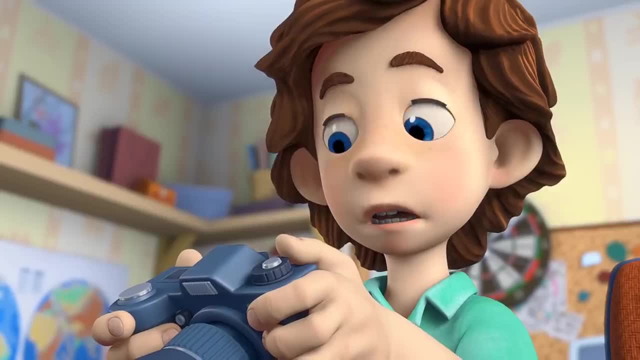 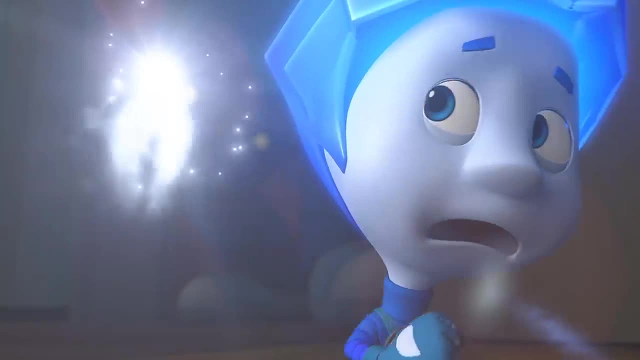 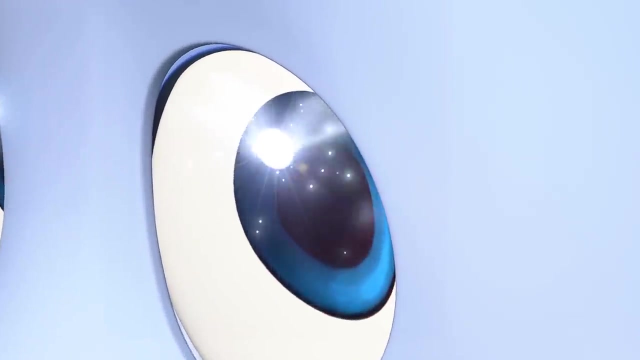 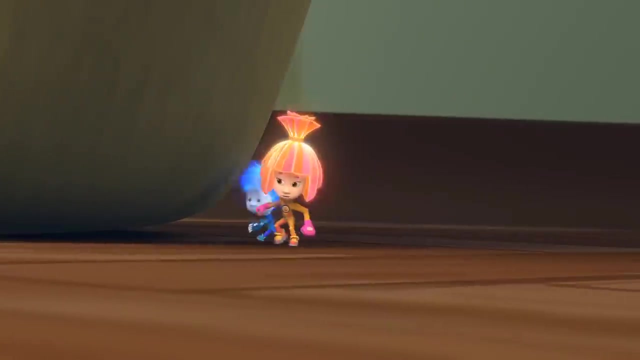 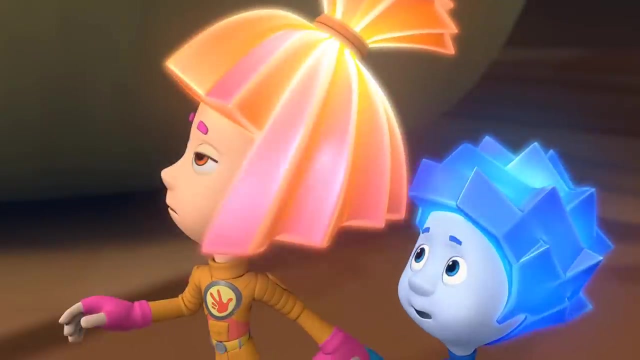 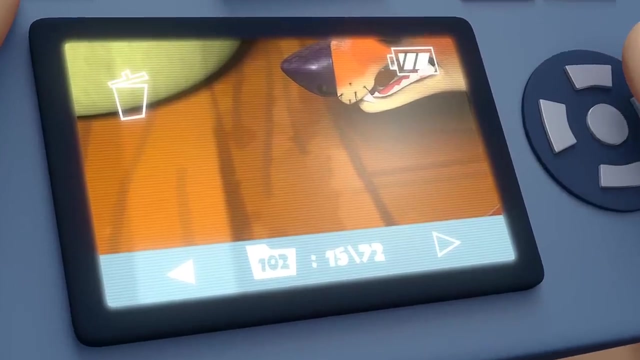 Nolik, let's run. You can't run from me. What happened? Where are you going? Chisaka? I've got you The story of the century: The monster and it's prey. Help. No, he won't help because he's a paparazzi. 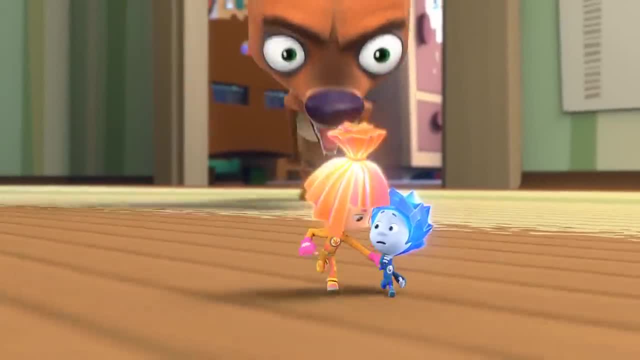 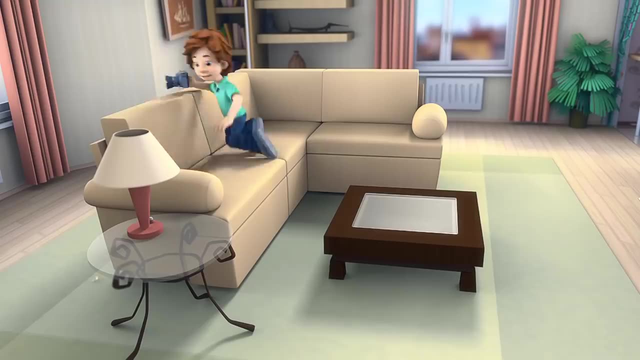 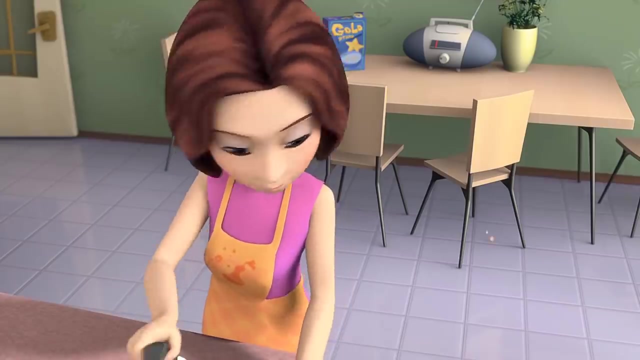 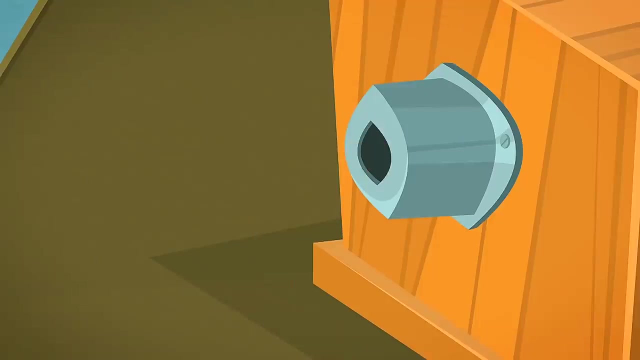 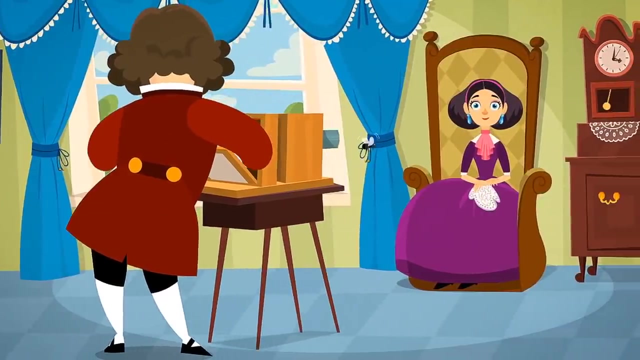 Yes, I got it. That's my best photo yet. What's all this noise about? Awesome shot. The first cameras were invented almost 200 years ago, but they worked very slowly. If you wanted to have your portrait taken, you'd have to sit still for a whole hour. 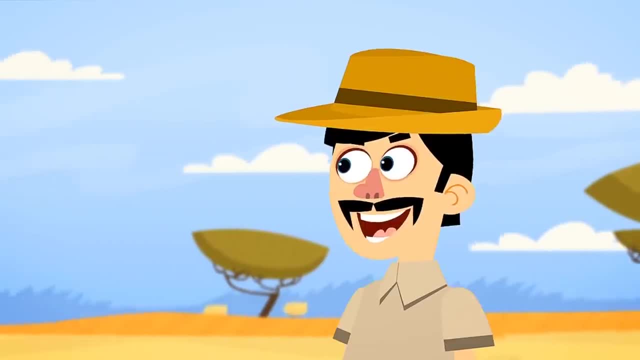 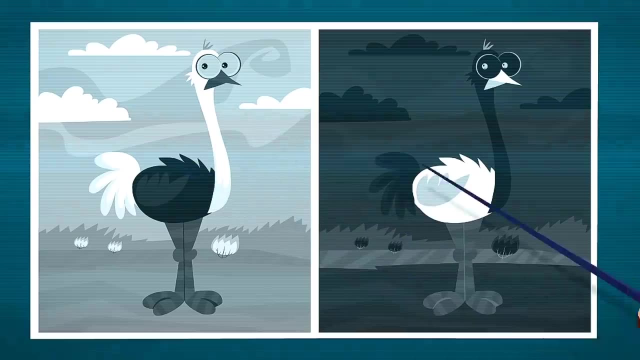 After film was invented, cameras got much faster and it became possible to take about 10 pictures a minute On a piece of film. everything appears to be backwards. Black parts of the picture are white and the white is black. It doesn't look normal until the picture is transferred from the film to a piece of 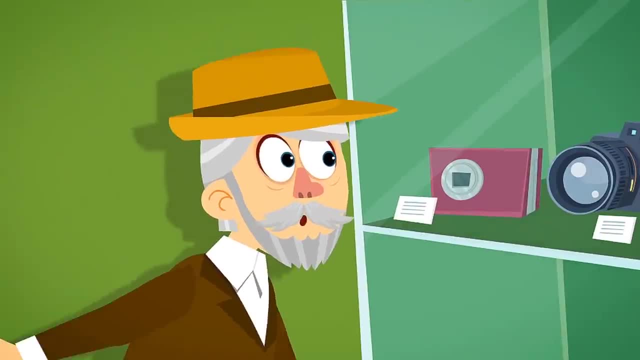 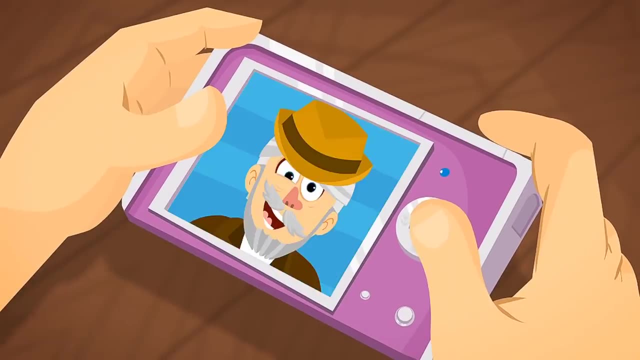 photographic paper. Now people shoot pictures with digital cameras that work without any film at all. You can look at what you shot instantly on a screen to see if you like it, And if you don't like it you can try shooting another one. 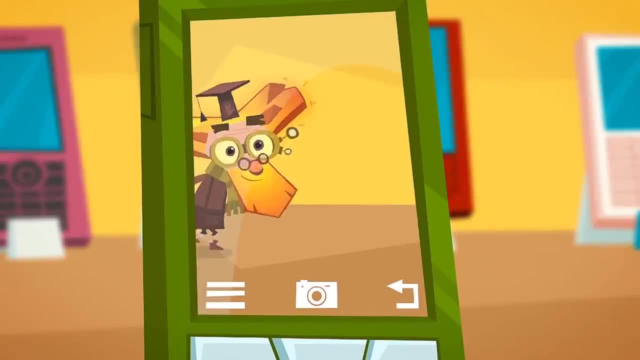 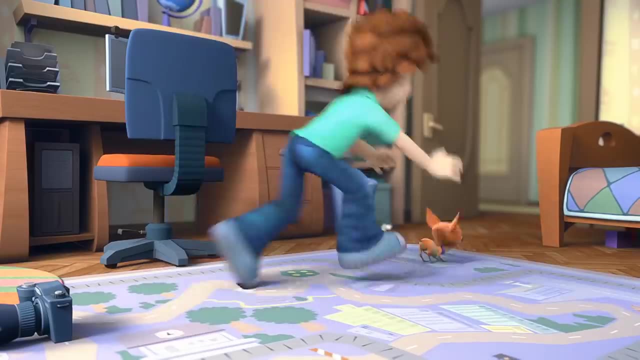 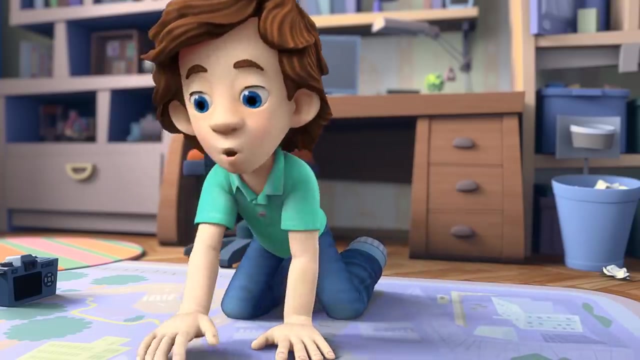 And today you don't even need a separate camera to take pictures. Almost every mobile phone has one. Oh, Oh, Oh Oh, Simka, Nolik, are you in there? Hey, come out, I'll stop shooting photos of you. 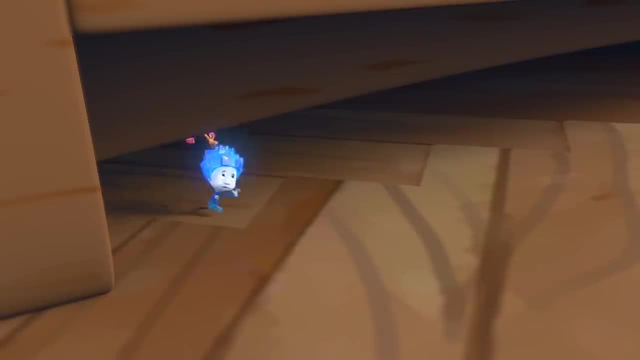 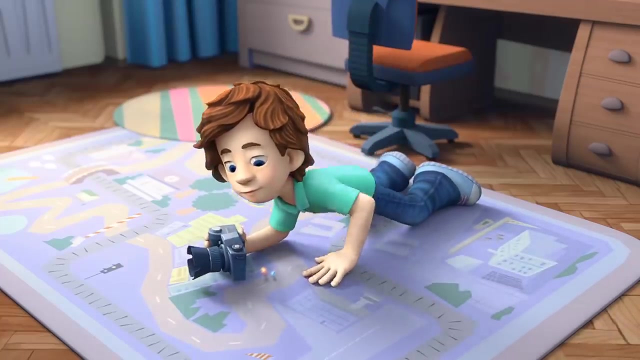 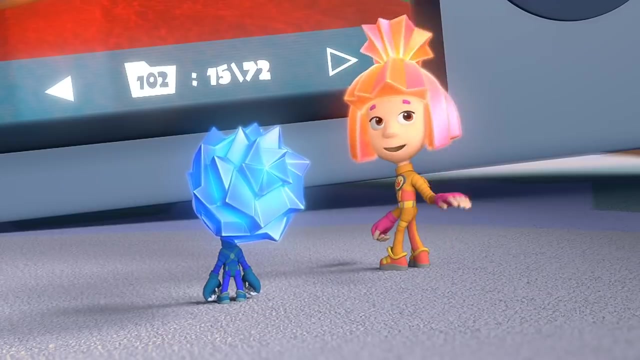 Aren't we friends? I'm sorry guys. Well, your friends were almost eaten alive by a dog. Please forgive me. Want to look at the photos I took? Heh, heh sure, go on, Show us what you got. 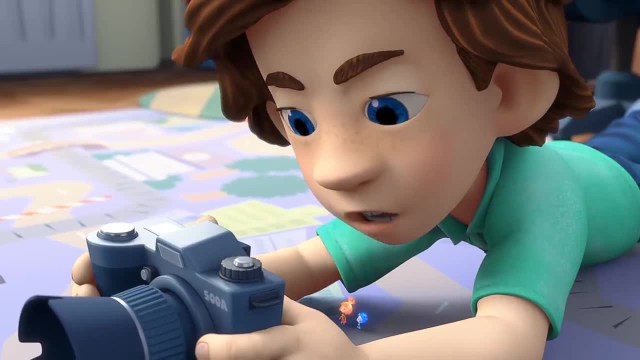 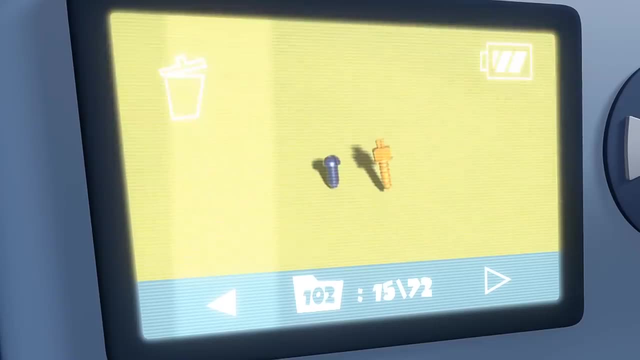 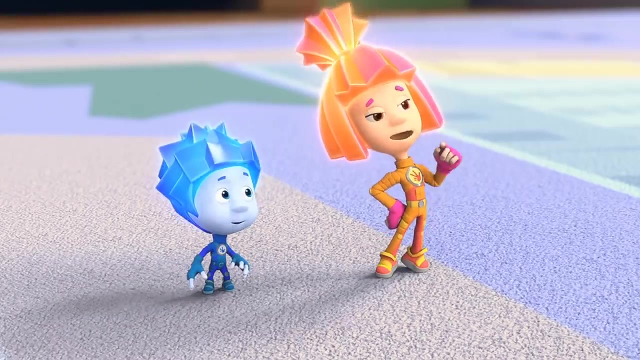 We're not in that shot. We're not there either. Ha, Well, done there, paparazzi it, I know for sure. look, I'm zooming in. it's impossible. I don't believe it possible. but when did you have time to turn into screws the same time you were? 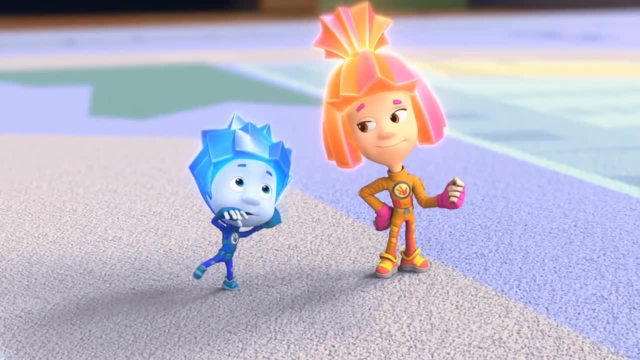 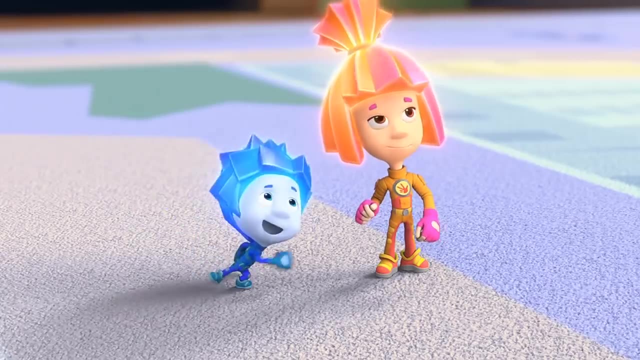 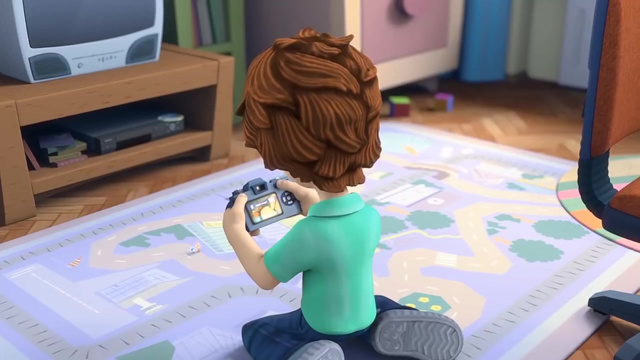 pushing the button. we're scared. we could change faster than the blink of an eye. you lost paparazzi. and what are you gonna do with your millions? mr paparazzi, would you please stop calling me that. you got it after every one of those photos is thrown away. all right, I'll delete them. and do I have to delete? 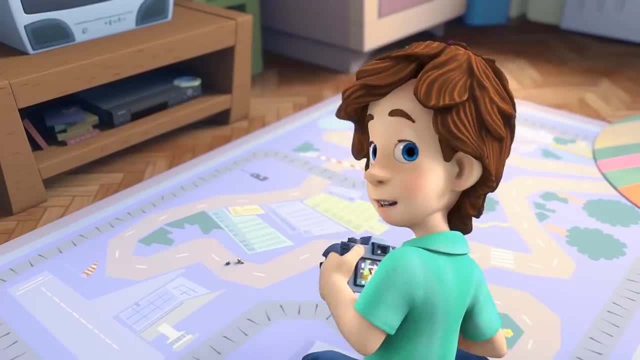 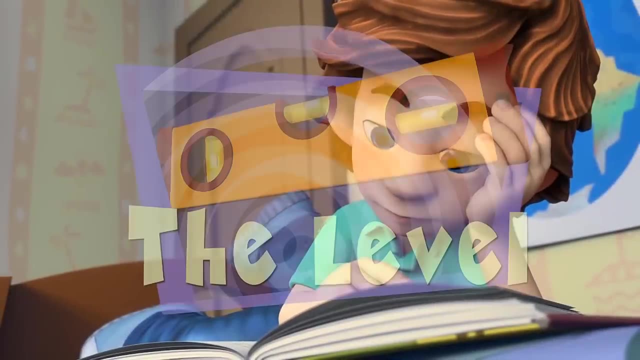 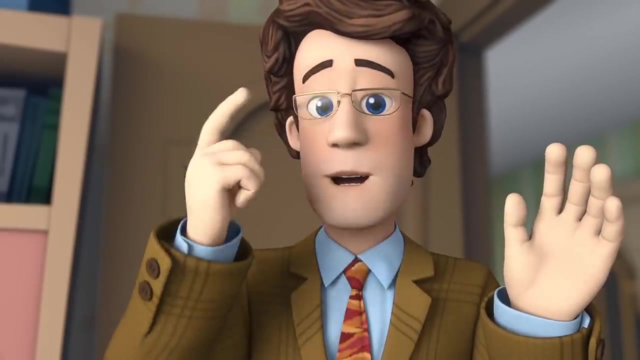 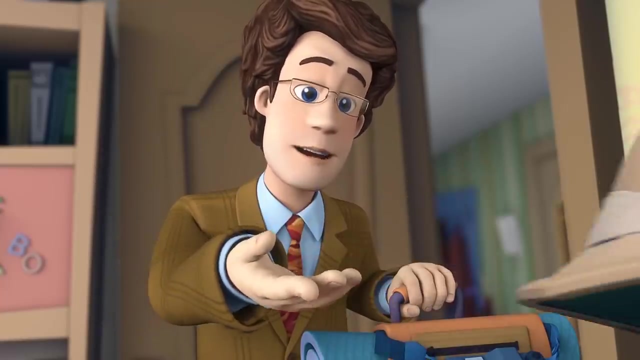 this one too. no, keep it. it's a great shot. I never even saw you take it the level. Tom Thomas, I'm really sorry. the movie this weekend I have to cancel. you do? I need to go to Africa for work? I leave tomorrow, oh cool, you think I could go with you to Africa? can you even find it on the map? 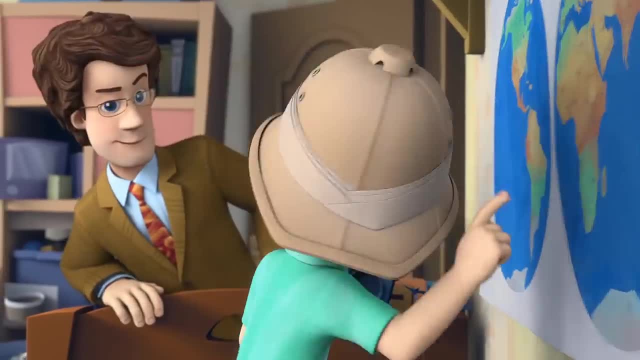 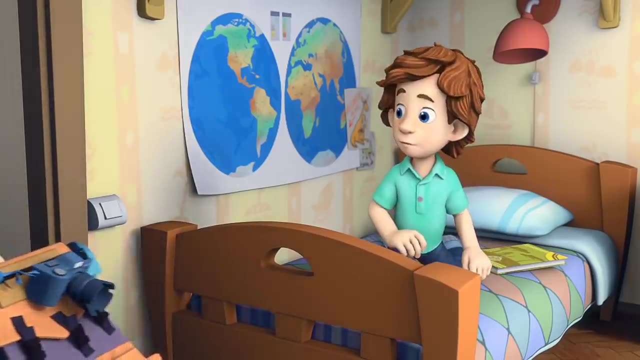 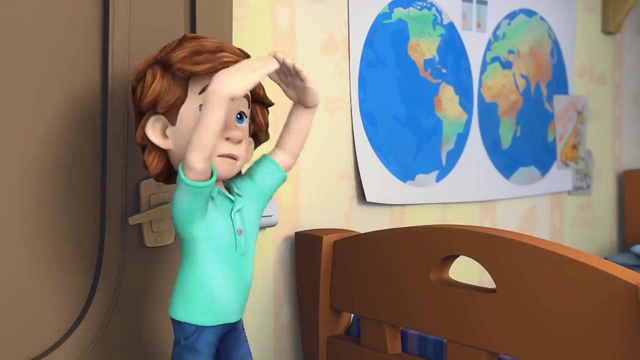 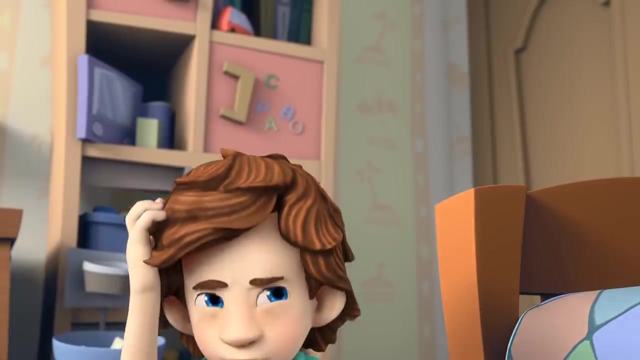 Africa. here we go, mm-hmm. no, you're still too little. when you grow as tall as the top of Africa, then I'll take you with me here there, Oh Thomas, what you're doing down there. I want to know if I'm as tall as the top of. 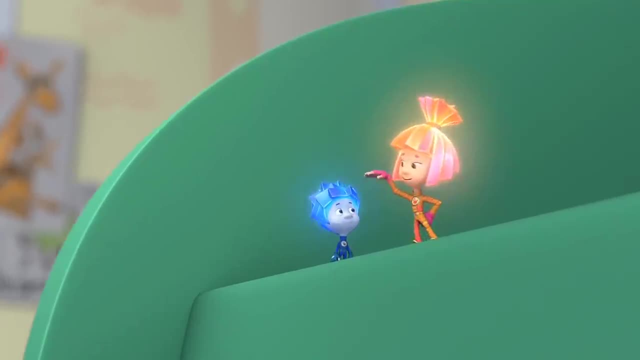 the Africa. well, do you know your height? okay, yes, Don Thomas, what would you doing down there? I want to know if I'm as tall as the top of Africa or not. well, do you know your heist like uh-uh? okay, then let's measure you and mark how tall you are. you just need to hold. 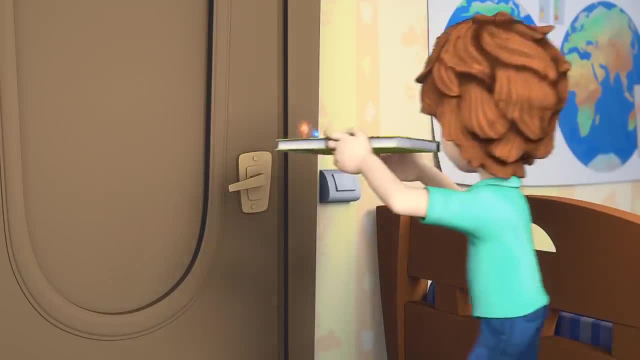 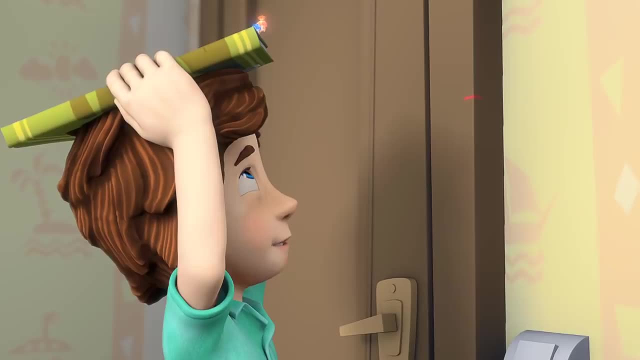 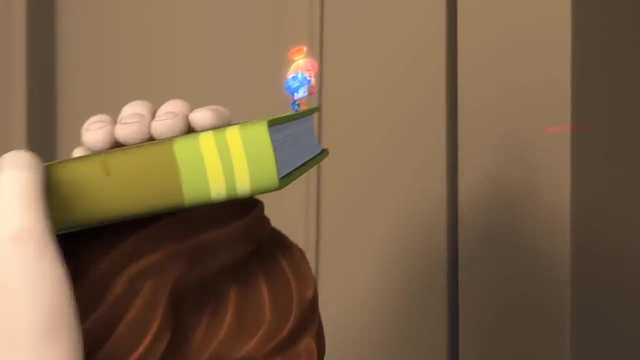 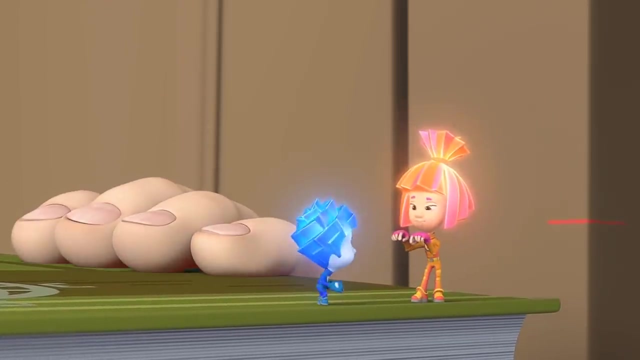 the book. all right me, Simka. how do we measure what's higher, the top of Africa or the slime over here? linear weights bound to that top of his. It's a tough one. We need a piece of flexible, clear tubing. Oh, I can get it for you. 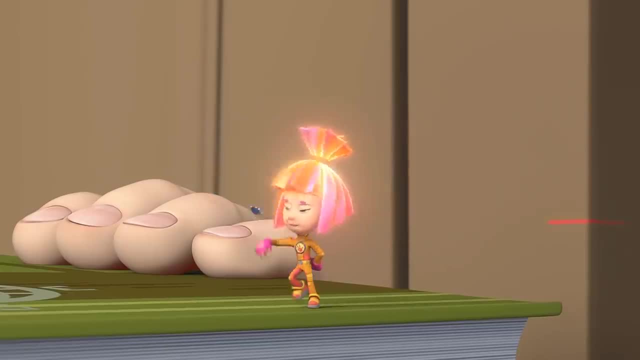 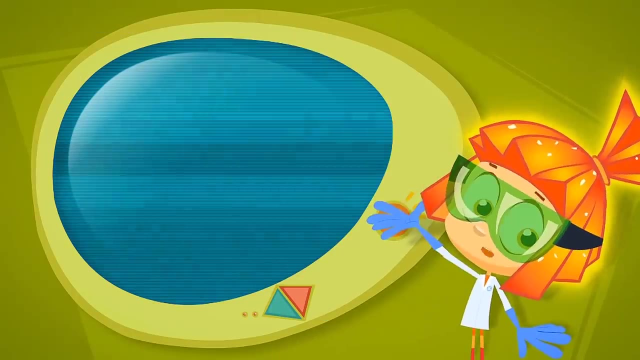 I know where it is And we'll build a simple tool to find out the answer. It's called a water level. Let's do an experiment First. we'll pour water into two bottles: A little bit more into one and a little less into the other. 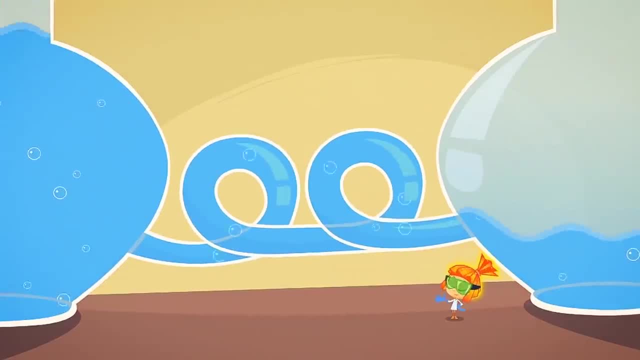 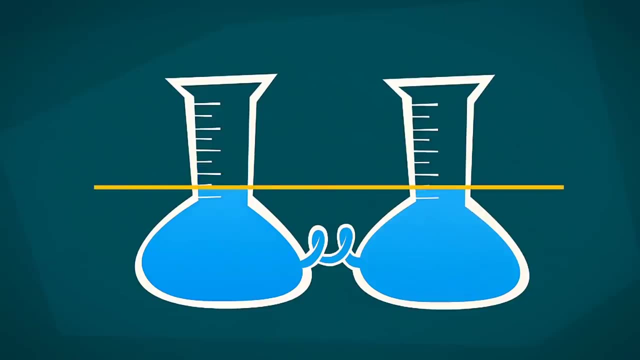 Now we'll connect them with a tube so that the water can flow between them. You see, The water flows and flows And then it stops. It stops when there's the same amount of water inside of both bottles And if we do this with a simple tube. 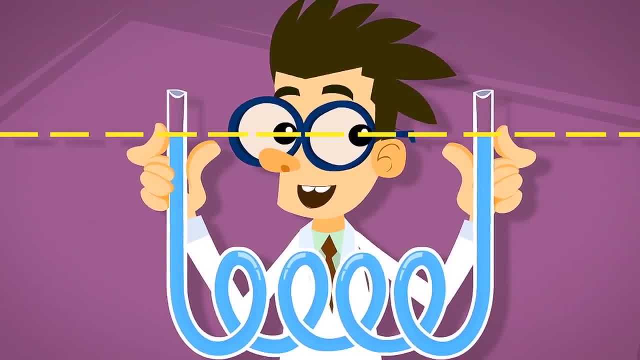 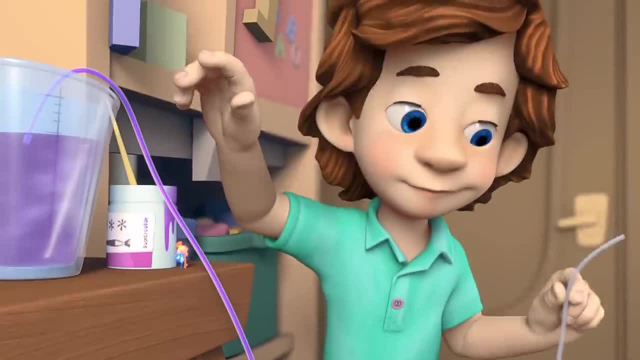 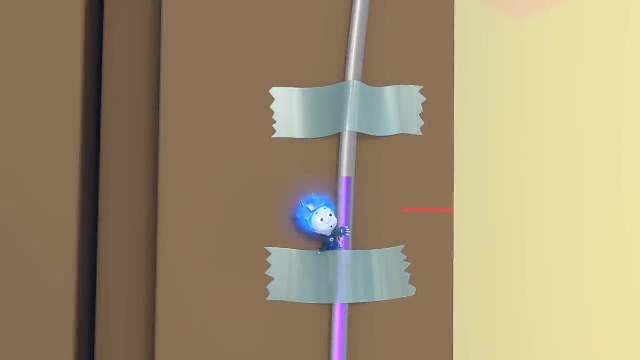 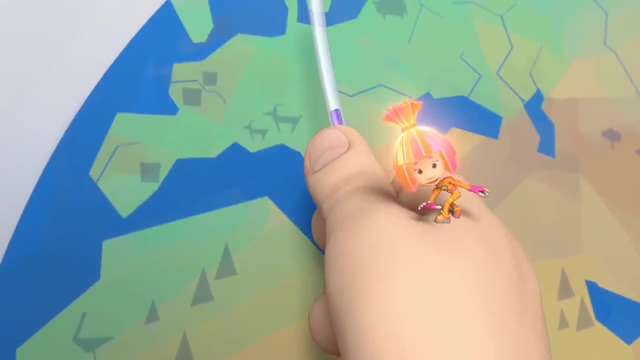 it becomes a useful tool called a water level, in which the water on both sides is always the same height. I'm going to watch the water level on this end. all right, Be careful how you lift it, or the water can get out. 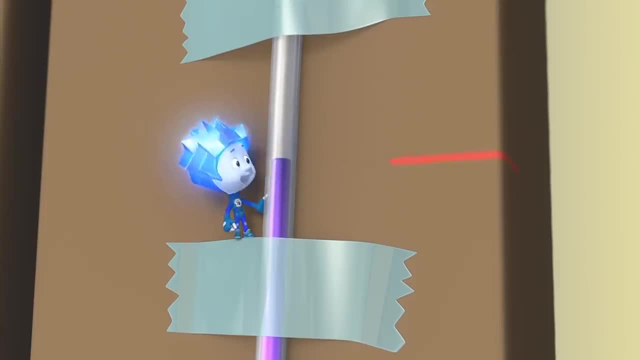 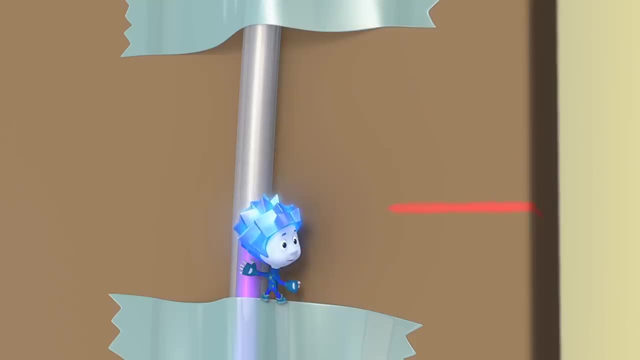 Nolik, what's going on? The water inside the tube is even with the line. There you go, Tom Thomas. Where the water is right now is how tall you are, And Well, it looks like Tom Thomas is going to be able to get out of the water. 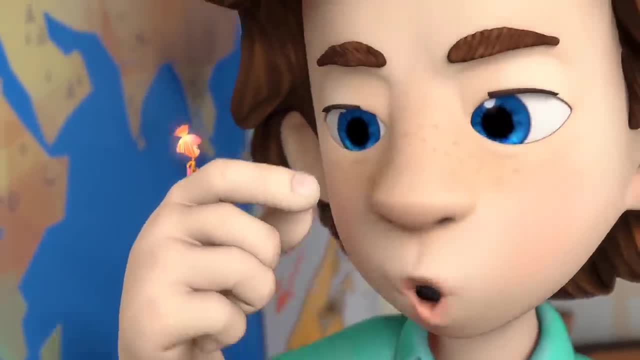 And Well, it looks like Tom Thomas is going to be able to get out of the water, But Tom Thomas isn't quite tall enough for Africa. What if we hold the tube a little higher? You can try if you want, but the water is going to stay where it is. 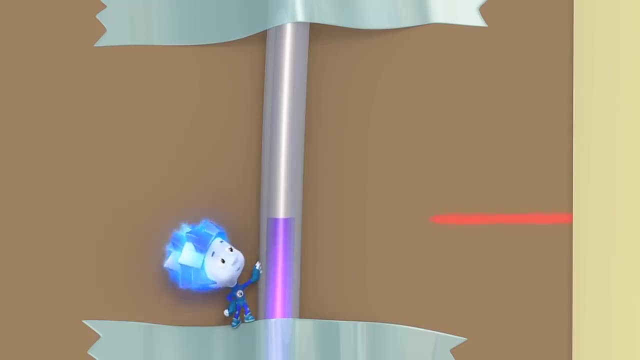 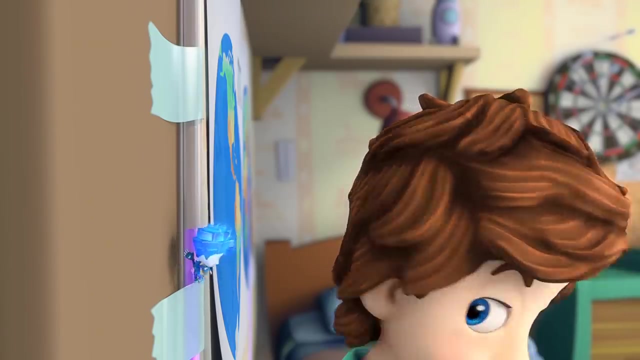 See, The water level on your side always stays the same as on the other side. I'm not getting that tall for a while yet. And what if we just lower the map a little? That wouldn't be honest, But it would be clever.